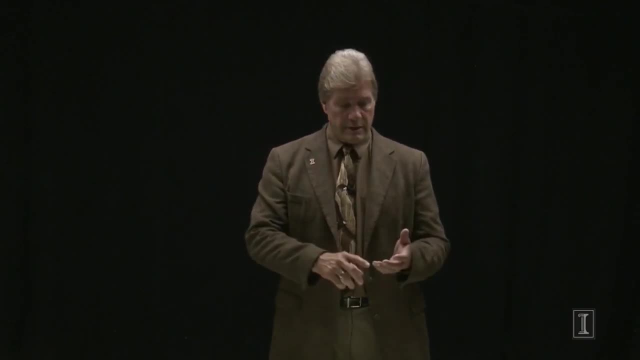 there. you expose it to the gamma. It kills the bacteria, it kills the fungus, it kills the viruses. You take it out and now it will have a much longer shelf life. There is a great example of this. Have you ever had strawberries and you left them in your refrigerator for a couple of 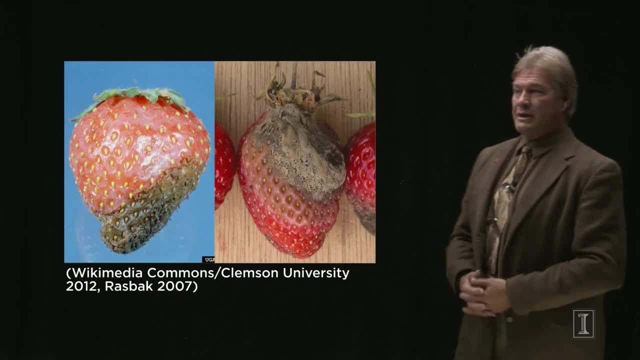 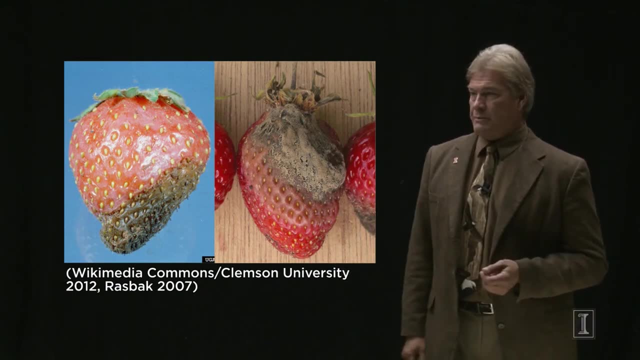 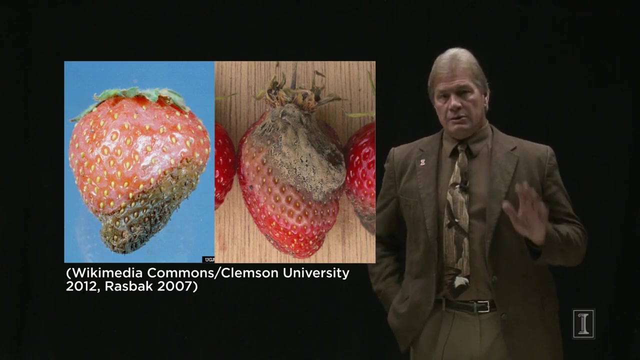 days. This is often what they look like. Very common It's a fungus, a mold, other things that grow on your strawberries. You don't want to eat that, So you buy them in the store. you better eat them right away. 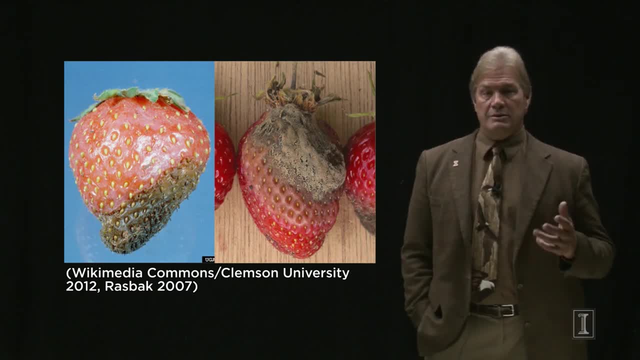 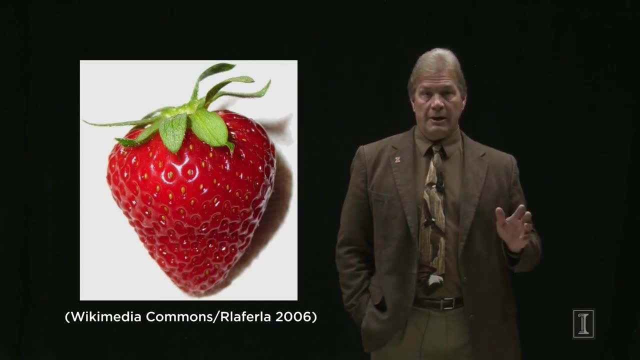 Stores can do various things to try to make the strawberries last longer, because, after all, this is the picture of the strawberry you want to eat. Now there are two choices. You could spray a bunch of chemicals onto the food, right. You could put on fungicides and mold removers and antibiotics. 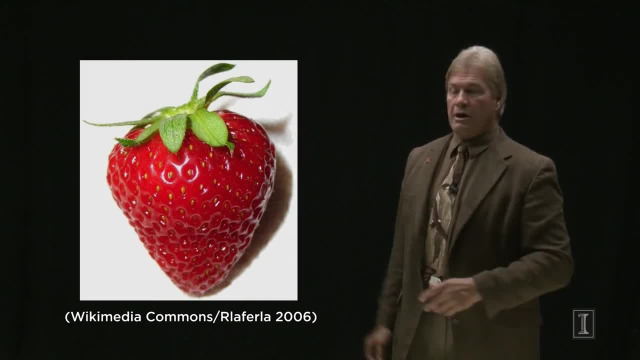 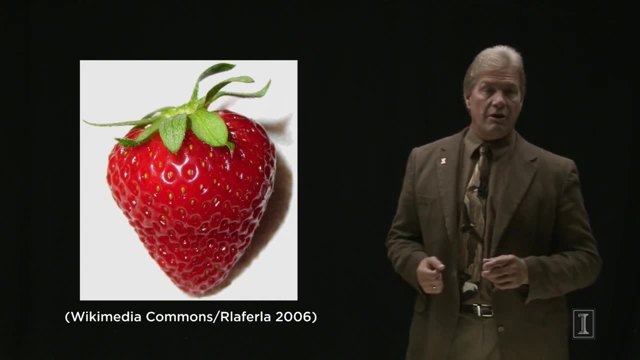 You have to be coating this delicious strawberry. Your mom always told you to wash your food before you eat it. Not a bad idea. Maybe you would wash it all off, or maybe it would just look so delicious you'd pop it in your mouth. 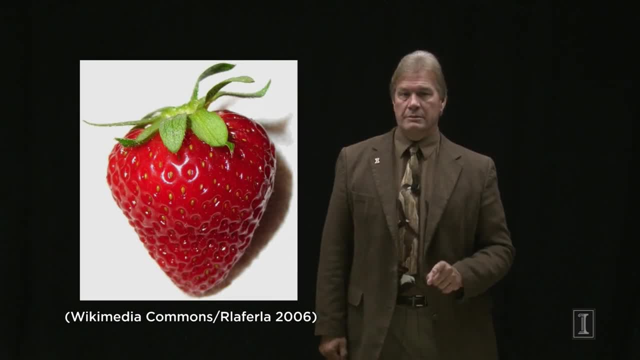 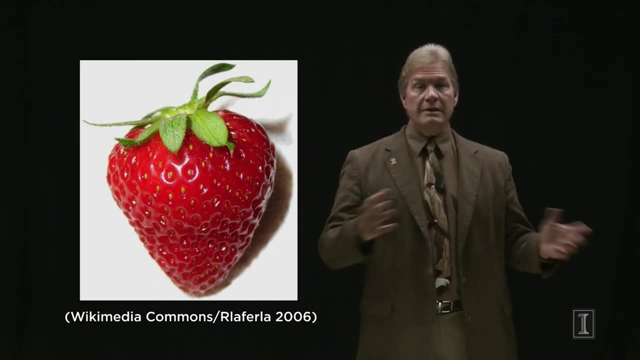 Or you could irradiate it. If you irradiate it, no problem popping it right in your mouth. The gamma rays killed the bugs. They didn't stay around. I'd much rather have a strawberry. I can't wait. I can't wait. 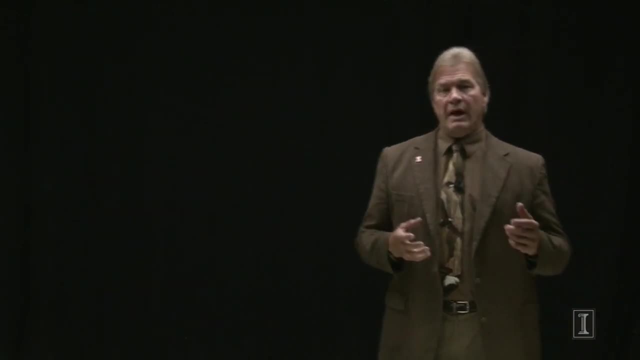 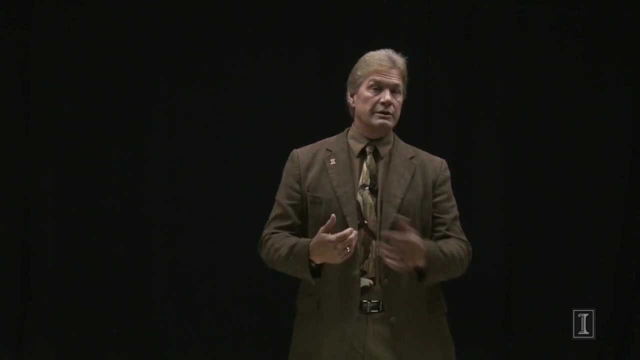 I'm not going to do an irradiated strawberry. So how do you know if your food's been treated with the chemicals which could be very bad if you ate them before you cleaned them off the surface, or if you had food that was sterilized? 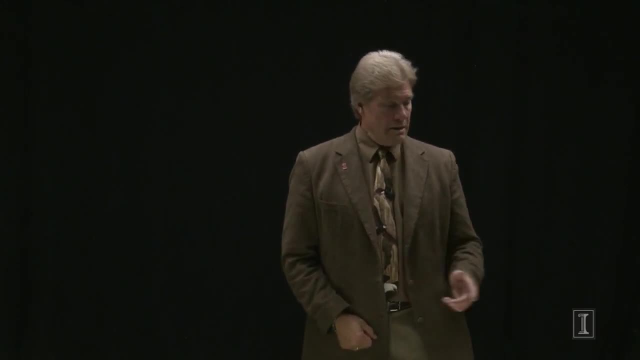 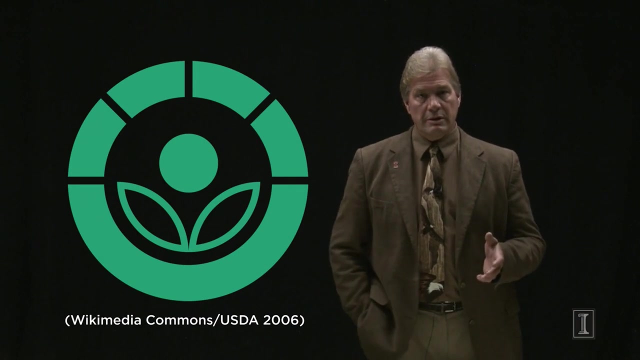 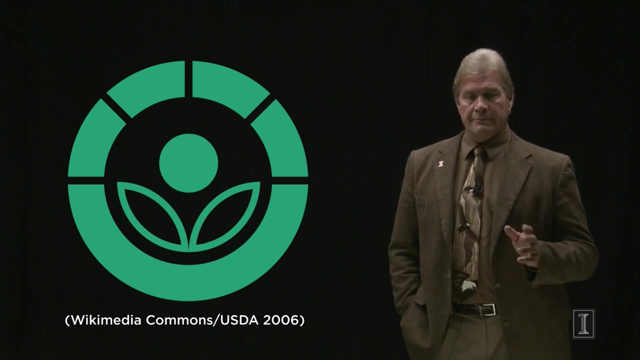 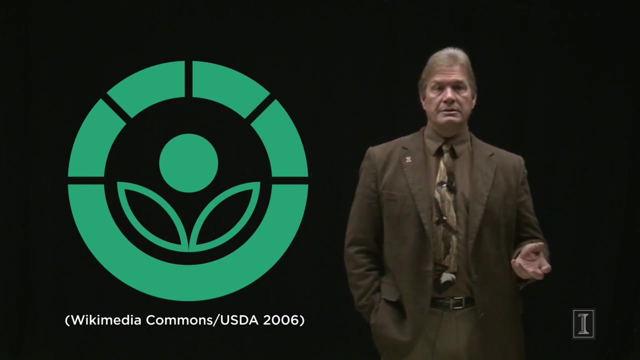 and kept with a longer shelf life by radiation. The key is looking for this symbol. This is the redura symbol. It indicates that things have been treated by gamma rays to kill off the unwanted bacteria and other items. Now there's always been the question of: does it alter the food in some other ways? 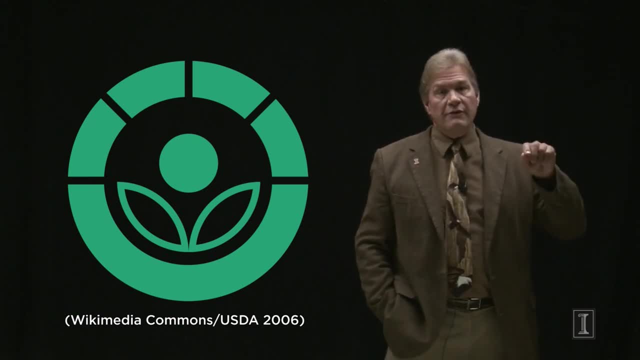 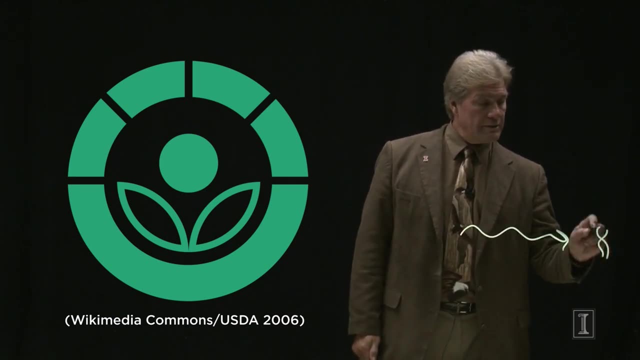 Are there negative consequences? After all, if you put enough gamma rays through, that can kill the bacteria, this gamma ray comes through. it's going to affect the DNA that's inside. here the bacteria is going to die. What about some of the proteins? 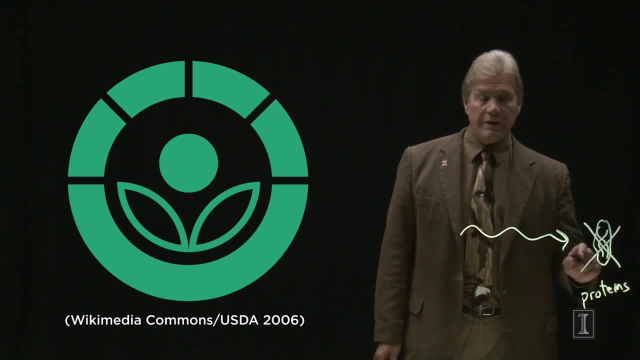 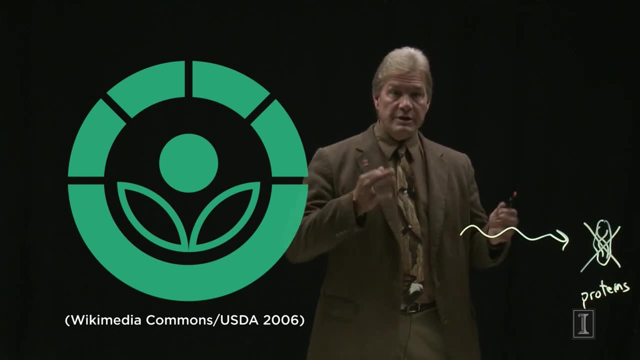 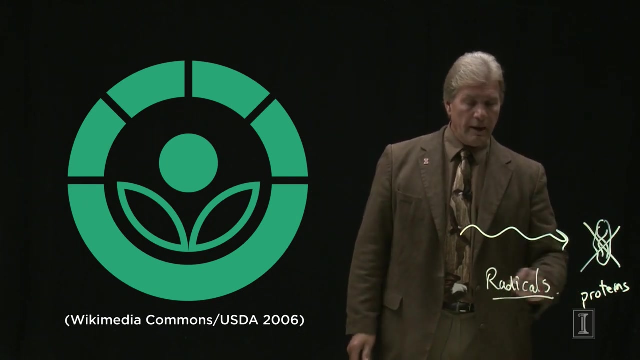 The carbohydrates, the other items that were in the food itself. won't it break some of them up? In fact, some people say, won't this make free radicals? Well, the answer is it will make some of those. Oh, free radicals are bad. 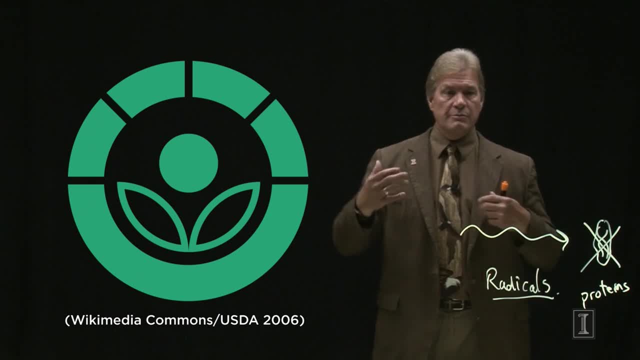 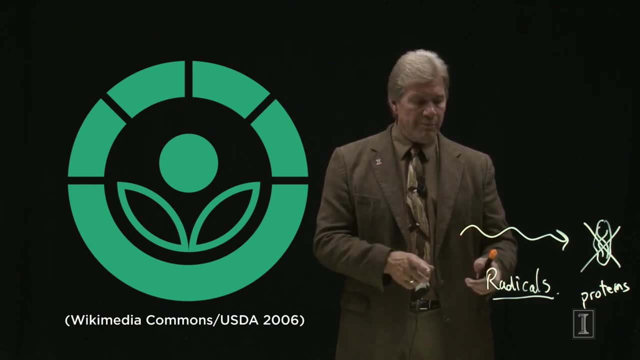 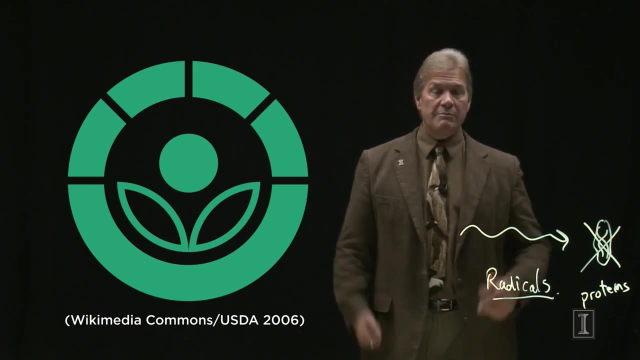 Well, they are very bad if they're in your bloodstream, if they're in your flesh, if they're in their body, They can cause genetic damage. But remember, you're going to eat this food. You're not taking the food and injecting it with a needle into your bloodstream. 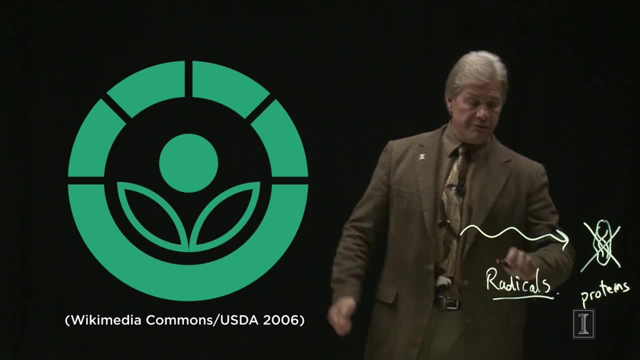 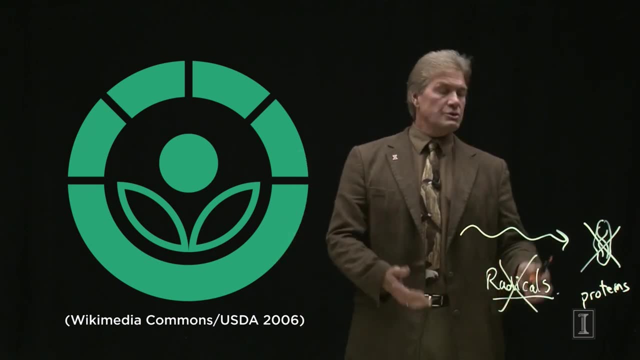 You're putting it in your stomach. Those free radicals aren't going to live through digestive systems and stomach acids and everything else. In fact, much of the food you eat has all sorts of broken up proteins and other things, because you cook most of it. 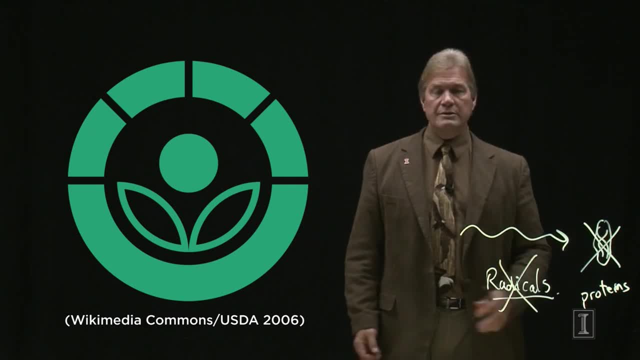 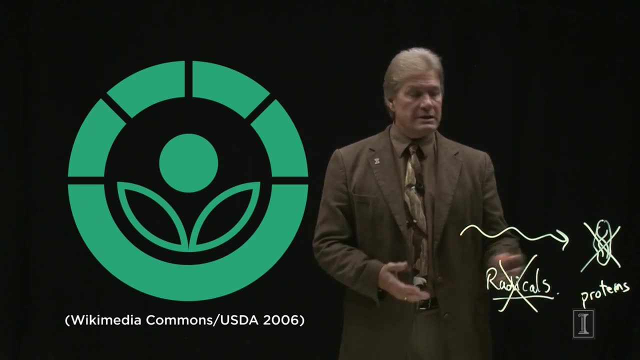 And in that process you make all sorts of radicals and other things too. But remember, you're going to eat this food. But when you digest it and eat it and chew it up and swallow it, this type of stuff, these quote negative consequences, the things that would happen to the substances in the 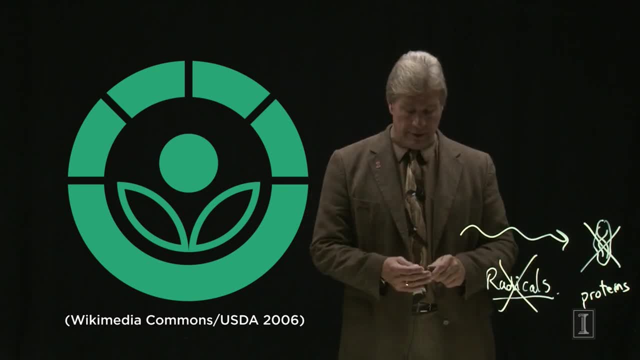 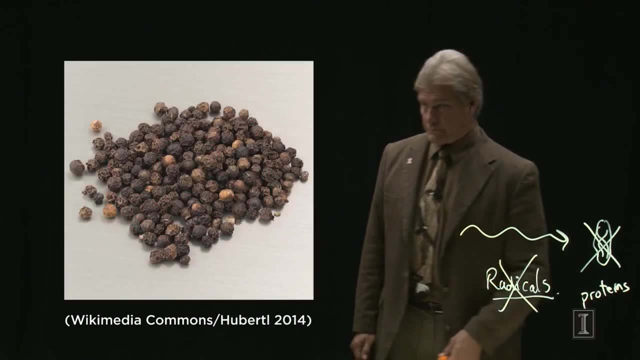 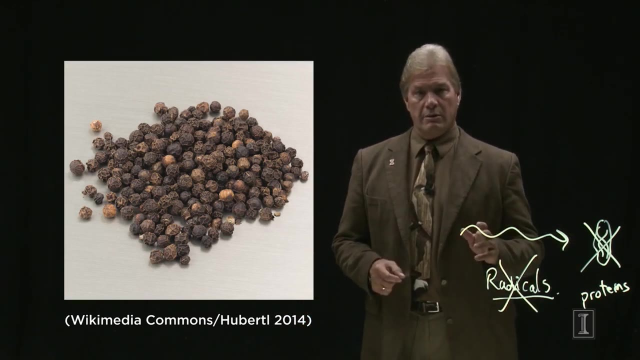 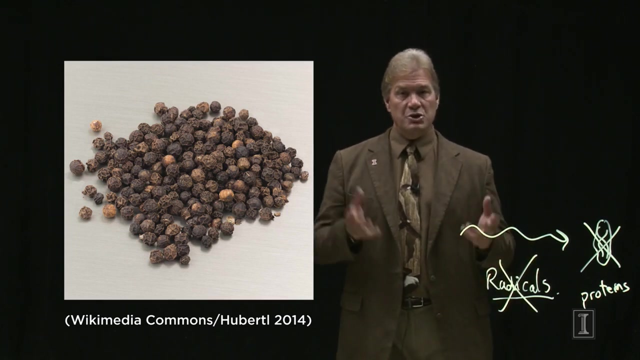 food from the irradiation. those are not going to be anything to be concerned about for your health. Another example: Virtually all the spices in the world Are irradiated first, Have you ever wondered why you can keep black pepper around on your shelves for years and 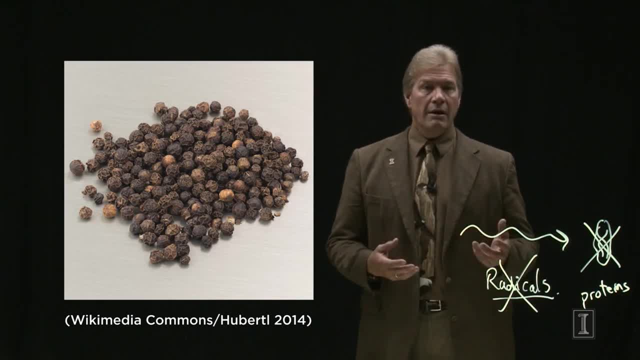 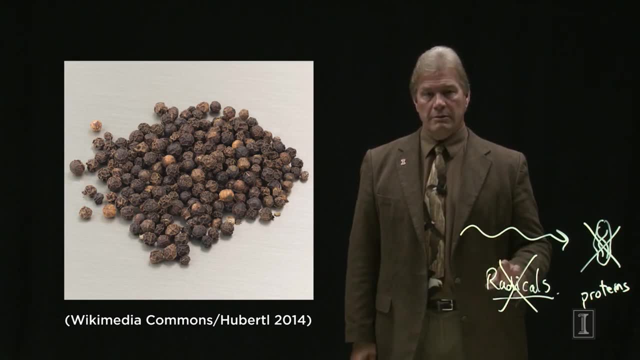 it doesn't all turn moldy or start rotting or have things growing in it, It's because it's been irradiated. It's fairly common and something that the public is afraid of but should not be. Hey, Let's go and actually see. 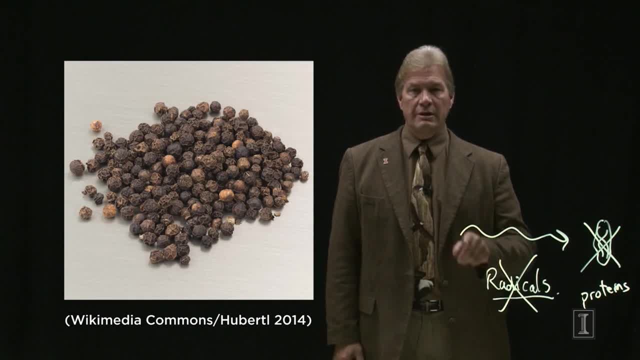 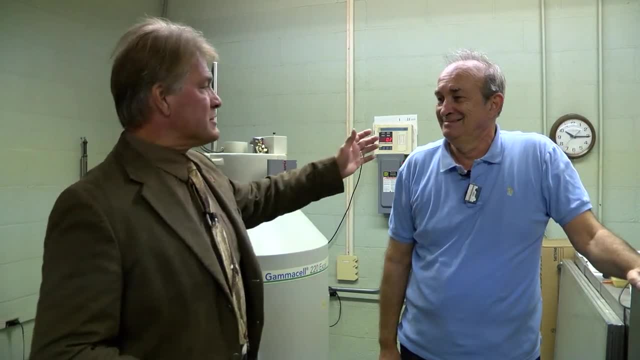 Okay, Let's go, Let's go, Let's go. Okay, So here we are. Let's go and see a food irradiator in action. All right, We are here today at the Nuclear Radiation Lab with my friend, senior research scientist. 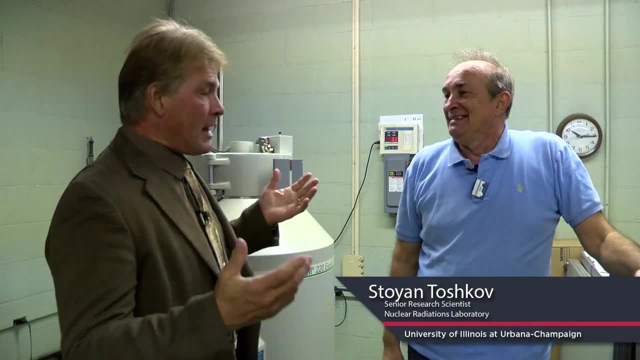 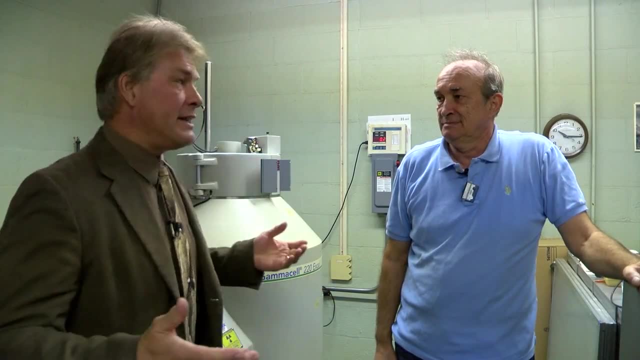 Stoyan Tashkov. Thank you for coming here. It's a pleasure. So we are here in his lab because he studies food irradiation and we actually have a food irradiator. So, Stoyan, can you tell us some about this device? 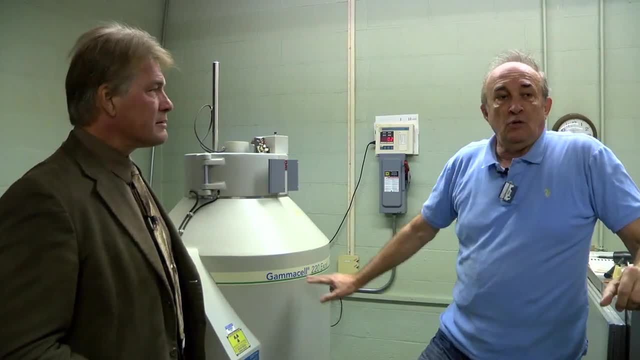 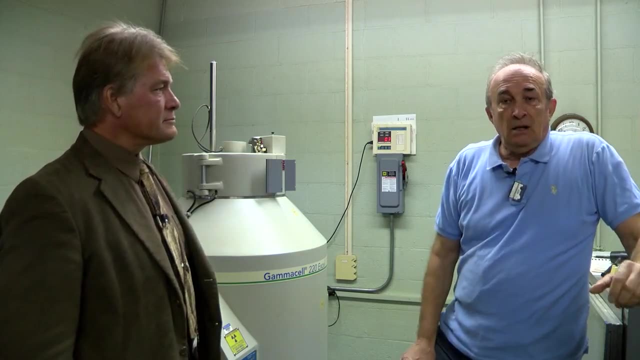 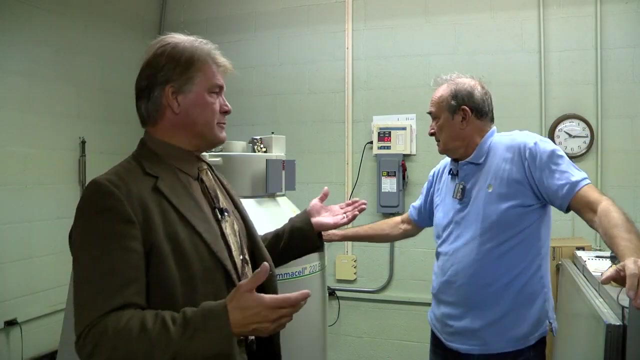 This is Canadian built machine Rode with two machines Rode with 24,000 curie. Wow, 24,000 curies Curie cobalt, Extremely safe to work, That's right. So our dose right here is just a tiny bit above background. 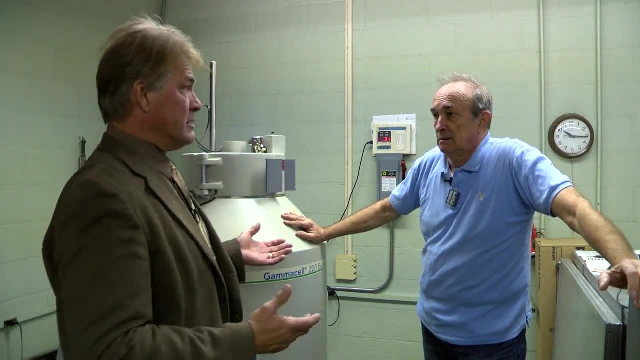 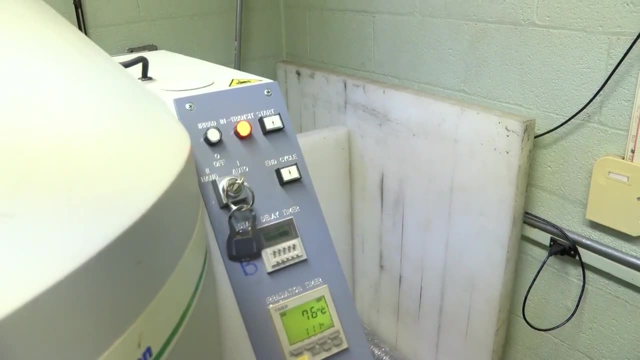 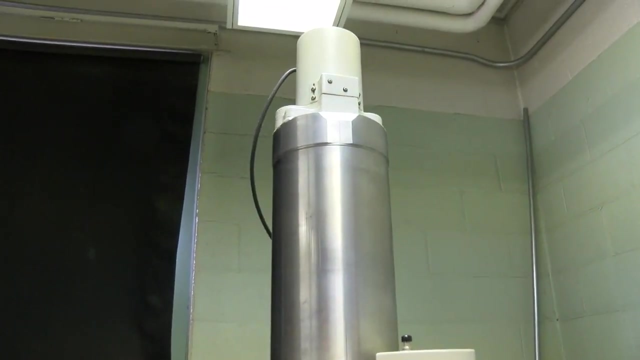 Yes, Right, And of course, inside the device where you'd actually be irradiating things, that is not some place we would want to stand Going up. So what we have here is you're actually raising the shielding right. 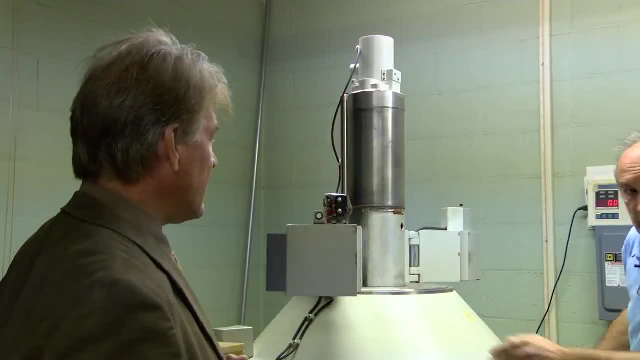 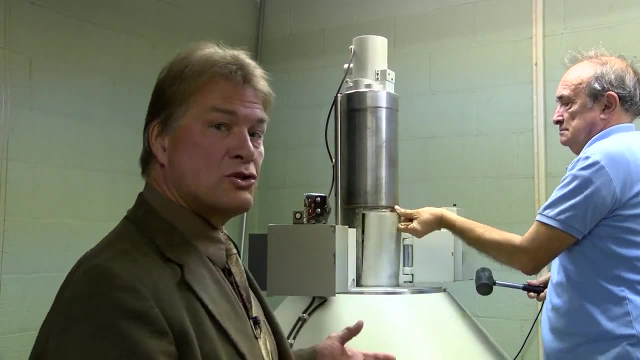 Yes, Okay, The radiation chamber, Irradiation chamber. Okay. Now you might say, oh my gosh, we're all getting irradiated. But that's not the case. The radiation source is still down inside the chamber, where it's very safe. 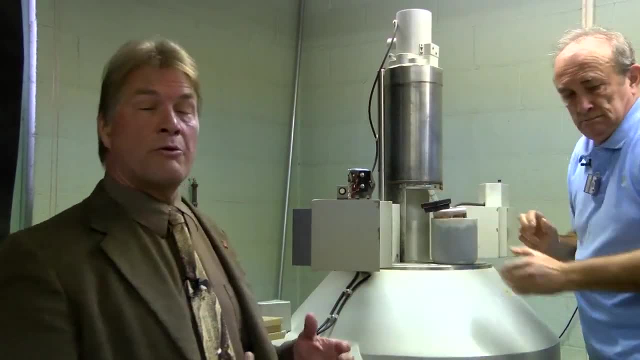 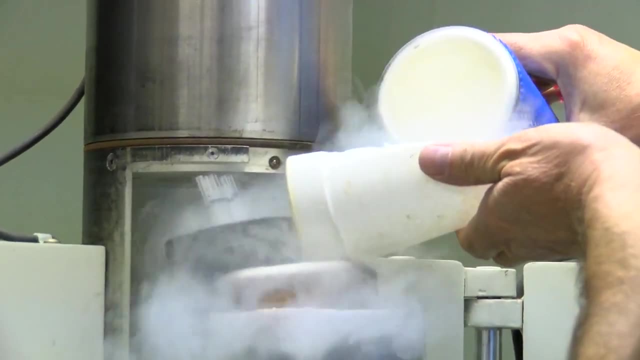 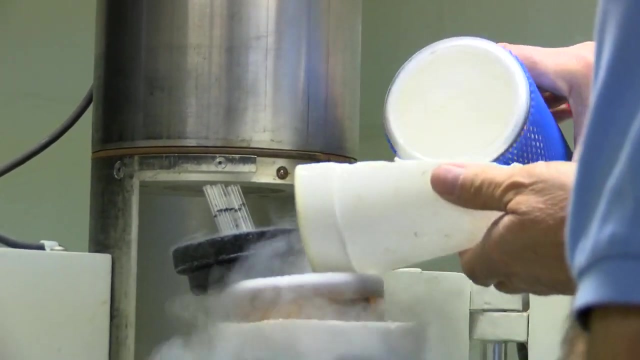 What we do is: this is the chamber where something would get irradiated and then you put it back in. So Stoen's adding liquid nitrogen, because in studying the effects of food irradiation it's important to separate that from temperature effects. So if you can keep things frozen, then you can see what will happen. not because maybe 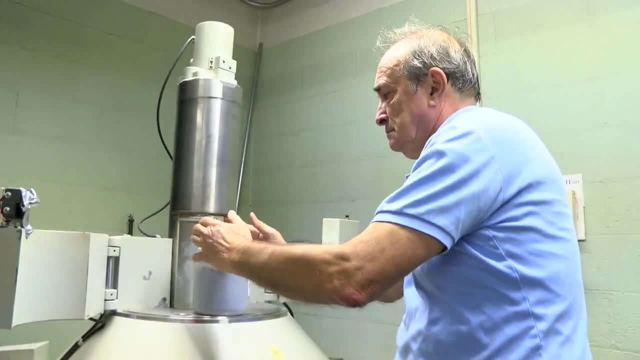 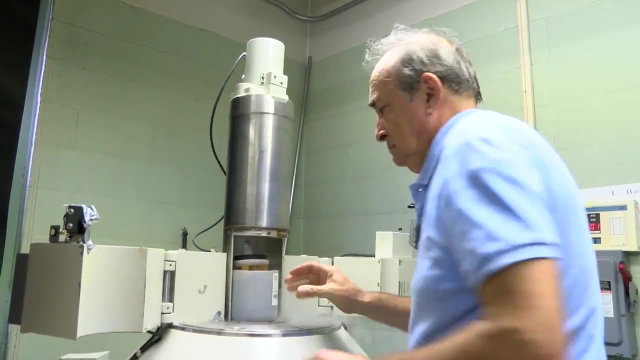 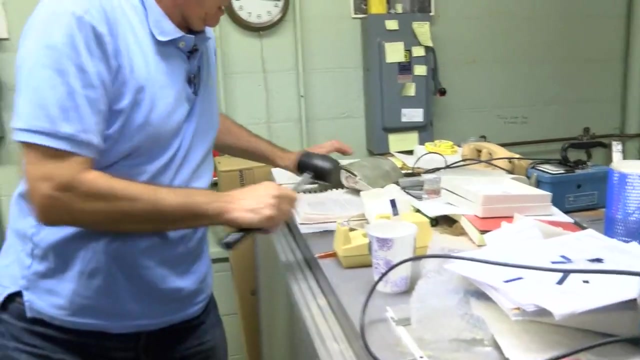 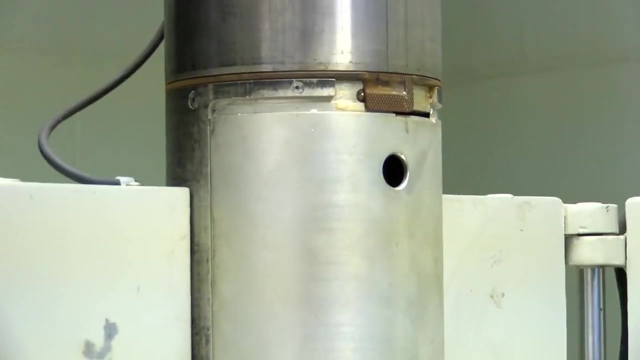 they got warm, but because they were actually hit by the gamma rays. Is there anything in there besides the liquid nitrogen? Any samples you're researching? Yes, yes, yes, The samples are there. Okay, I'm going to close that and I will close the machine. 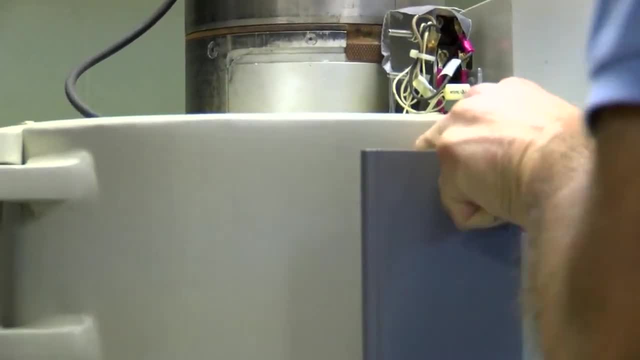 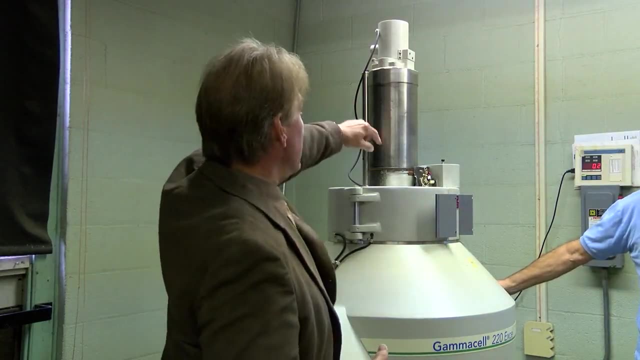 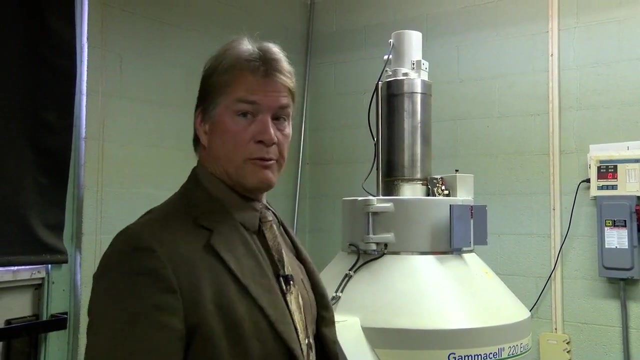 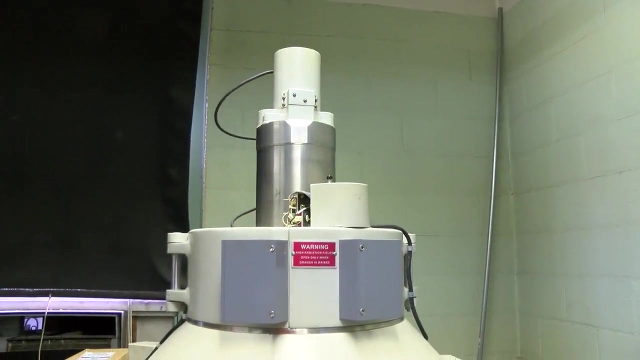 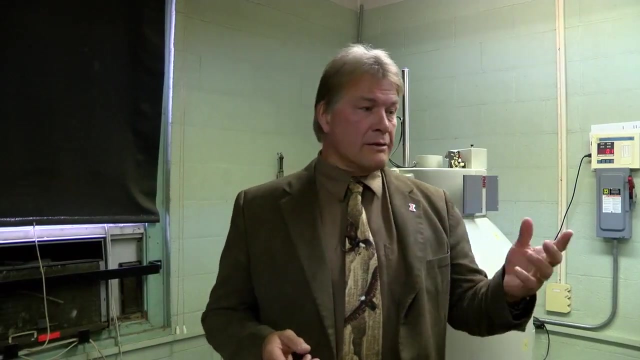 So now that's a sample that will be irradiated And again, our dose has never changed because the radiation source is inside, And now we put this and all of this shielding on top will go back into the irradiation chamber. I think this is a particularly interesting example. 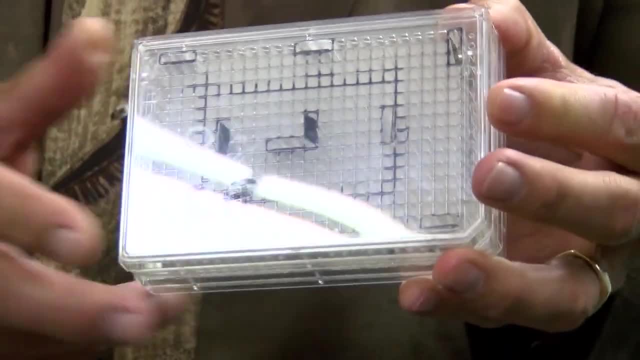 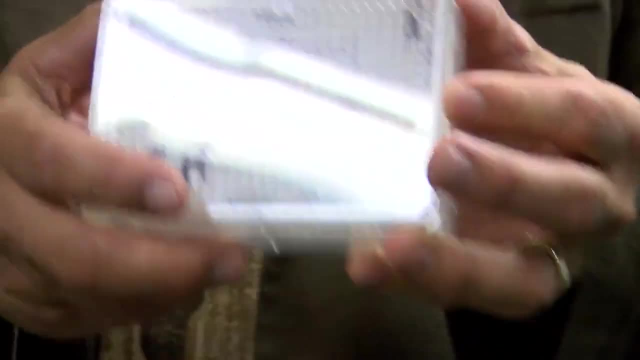 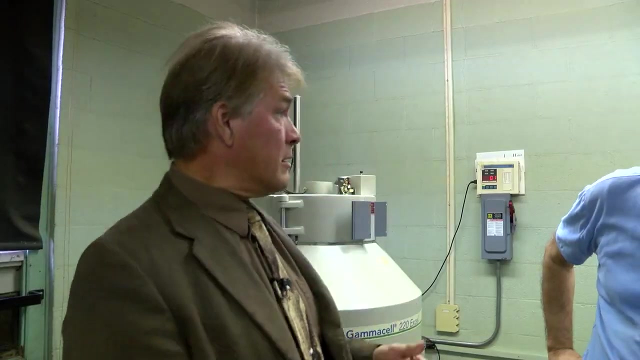 Here are a variety of medicines And, if you might imagine, if you have cancer treatments and they're doing radiation on you, you might wonder: well, will the medicine you're offering be irradiated? Will the medicine you're also taking be changed because of the radiation treatment? 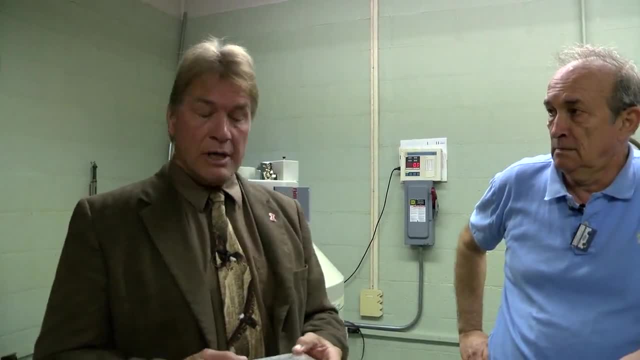 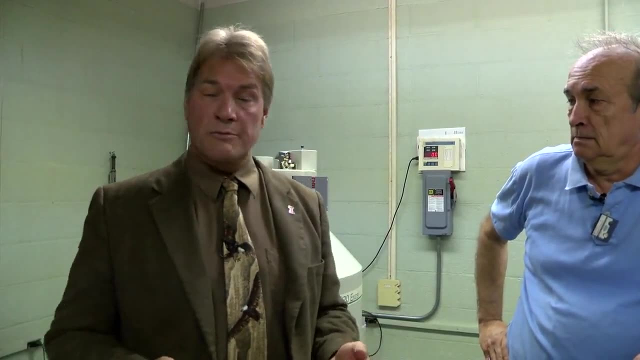 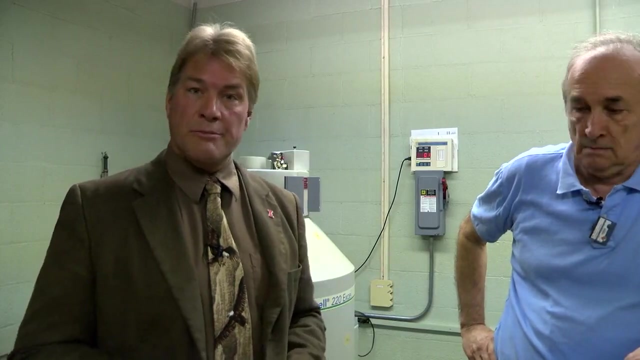 This way. one of his research projects is actually to determine that, because he can expose the medicine into a similar environment of a radiation treatment that a patient would have and then find out afterwards if the medicine has changed its efficacy and its use and its chemical composition. 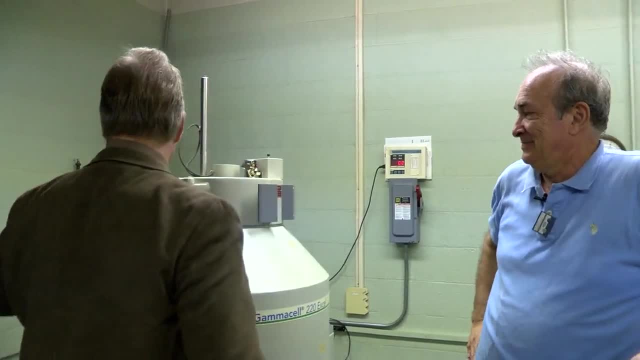 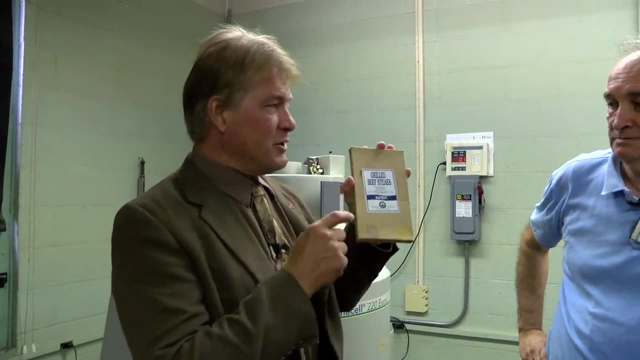 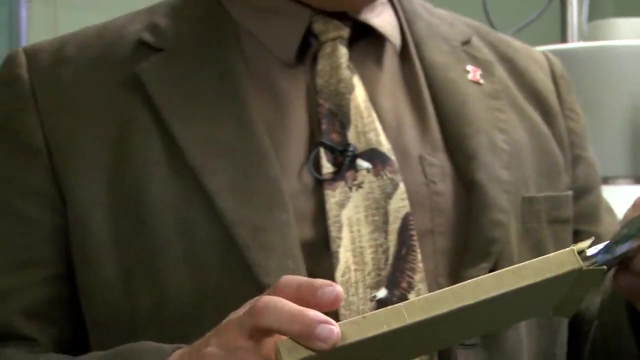 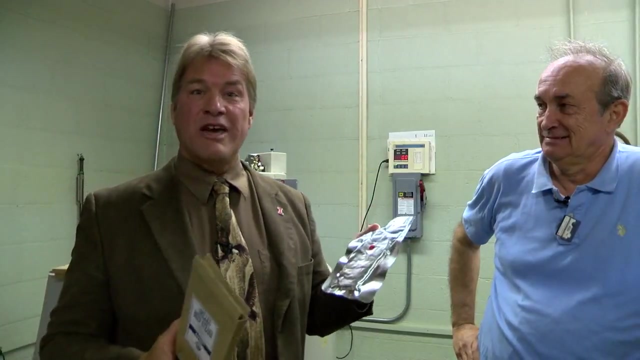 I think another one which you like showing off is the grilled beef steaks. These are supposedly delicious, right? Have you eaten one before? Yes, Okay, So these are what we send up in space with our astronauts, And it's very important that they don't get any kind of infection. They don't get any disease. They don't get food poisoning when you're up in a space capsule or a space station. So you want to make sure that the food has been irradiated so all the bacteria have been killed. It doesn't hurt the food. 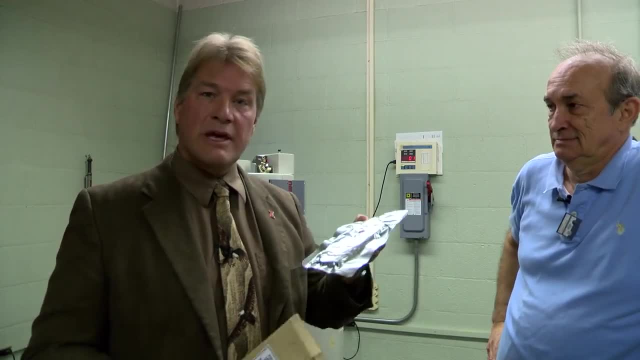 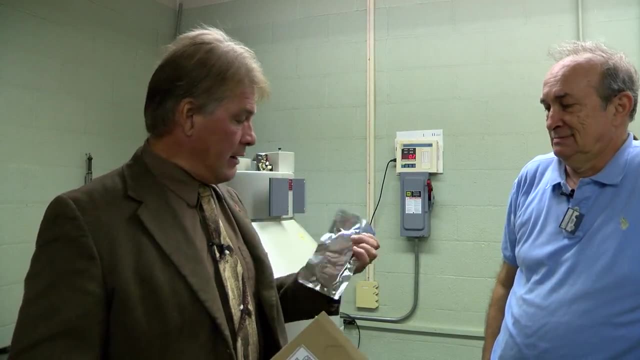 The food doesn't become radioactive, But what happens is that all of the germs that might be in it from processing, from the cow itself, get cleaned off, And you can tell, because this then turns a color. the radiation signal, Yes, Before radiation is yellow. 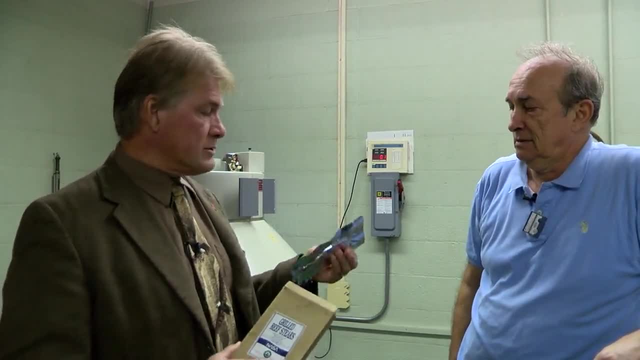 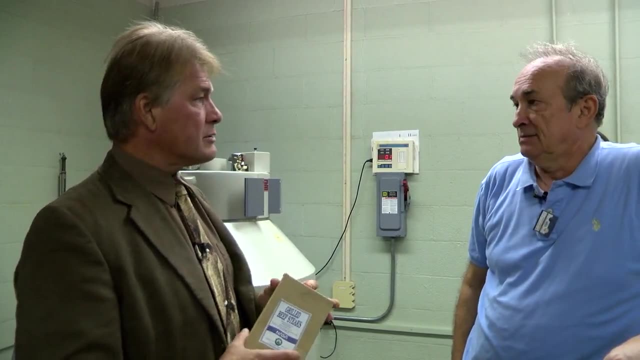 This is indicator, And afterwards it's red, And so this has no bacteria left alive in it And it becomes very, very safe to eat. And it's not just astronauts, right? Yes, There are people that have had transplants. Yes, In the Soviet time all the food of this around 5 million army Soviet Union used irradiated food. So the Soviet armies always used irradiated food to keep their. Now I don't know Right, We don't know now. But the key was that you don't want your troops to get sick- Right To get sick from eating bad food, So you might as well. One way to really sterilize it, and to do so without affecting the quality of the food, is food irradiation. 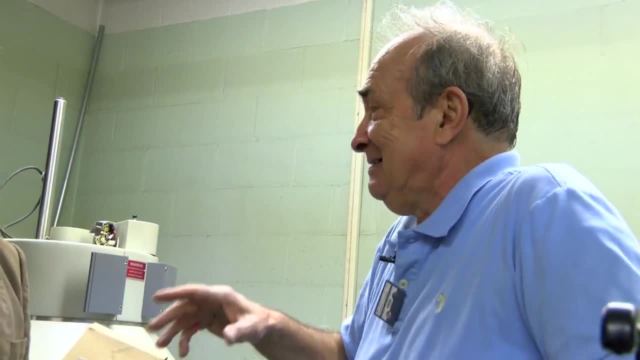 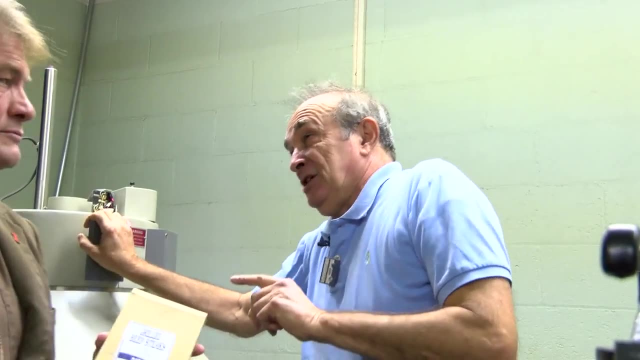 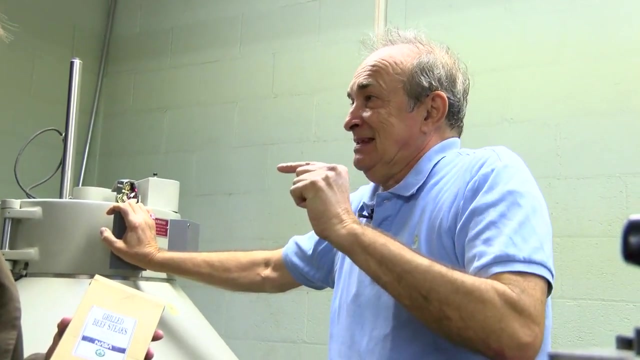 When we irradiate it's dangerous, But after a second the food is absolutely not radioactive because the energy is 1.3 MeV. Mm-hmm, Mm-hmm. So we start induced radiation. That means we are absolutely safe. Absolutely. A nice analogy of this is: if you shine a flashlight on something, it doesn't start giving off light. It's the same thing here. You hit these with gamma rays because it kills the bacteria. It doesn't mean this gives off gamma rays just like a thing that got hit by any other. 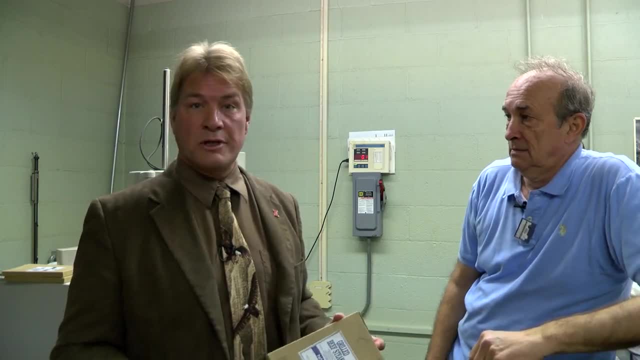 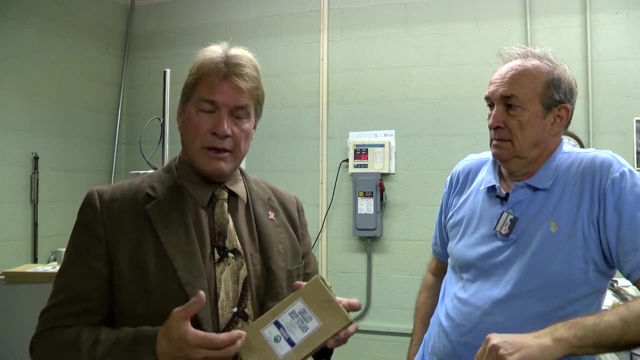 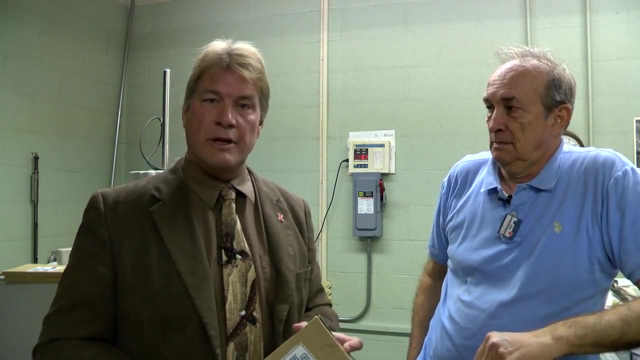 type of light? Yeah, After all, gamma rays are just very high energy light. So what we do when we irradiate food is we kill the bacteria, but then the food is not any more radioactive or different than it was before you put it into the food irradiator. 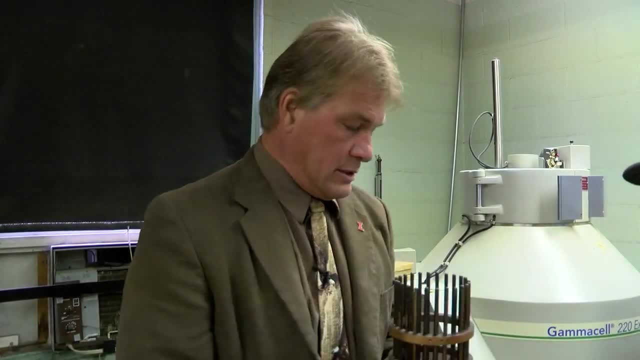 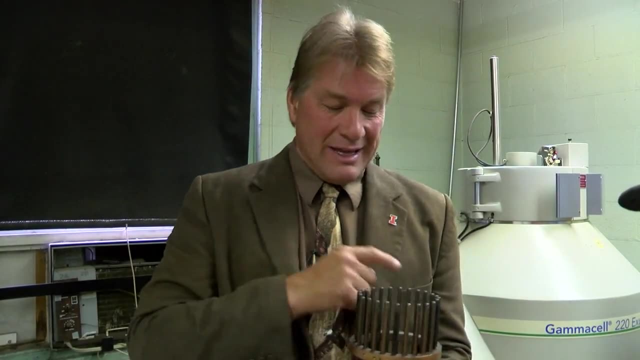 So what's actually inside this machine? This, Of course, this isn't really made out of cobalt-60, or I wouldn't be touching it like this, Okay- But inside there, each of these rods is actually a rod made of the radioactive food. 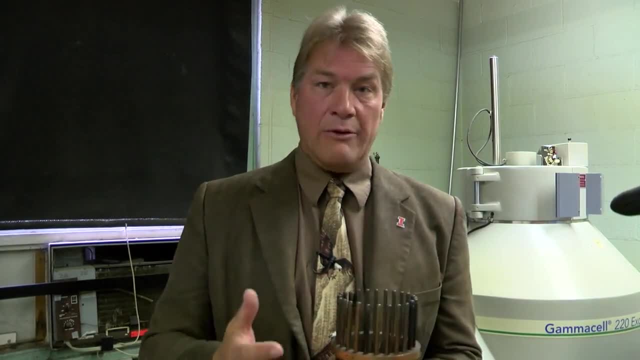 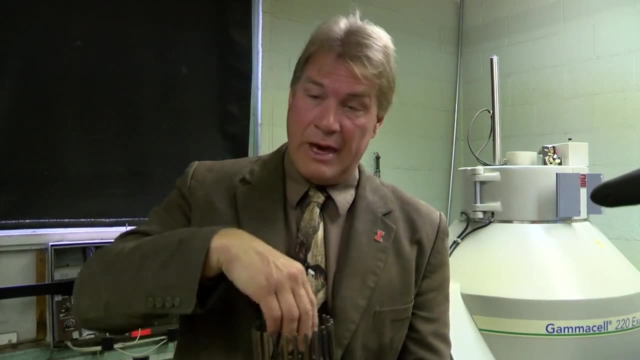 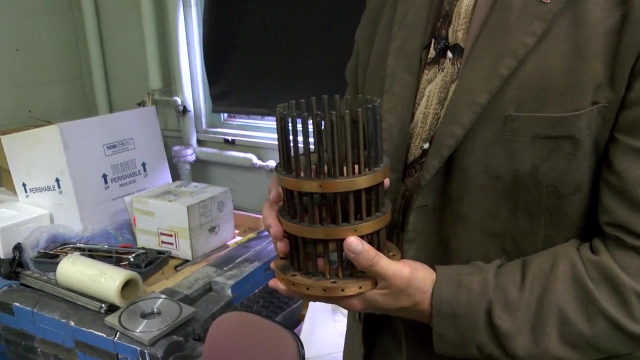 Okay, So what's inside this machine? This, This, This is the radioactive element, cobalt-60.. And therefore a sample: the food, the steak, the medicine. something else that Dr Toshkoff is testing is in this field, where all of these are emitting gamma rays. 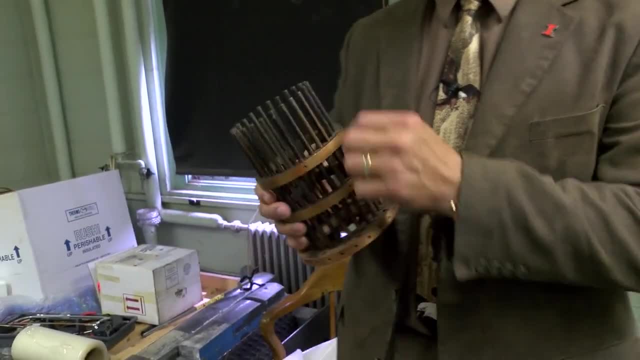 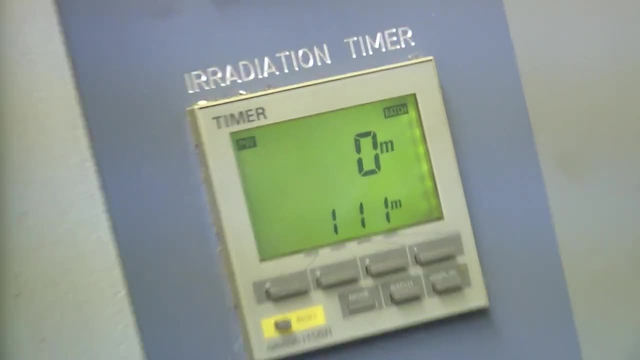 So this is really neat to see what would be the actual device. in here This is just made out of copper, but the actual thing would be made out of the radioactive elements themselves. The nice thing is this machine is foolproof. There's no way you can actually physically see it. 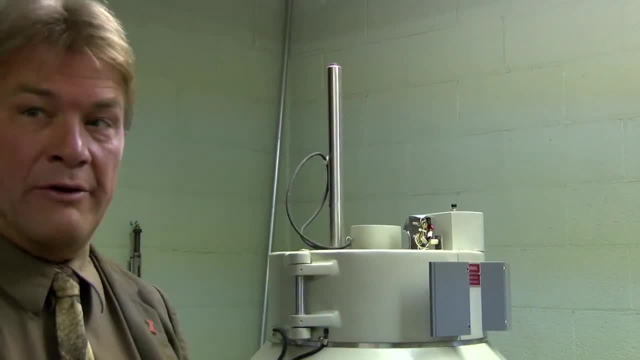 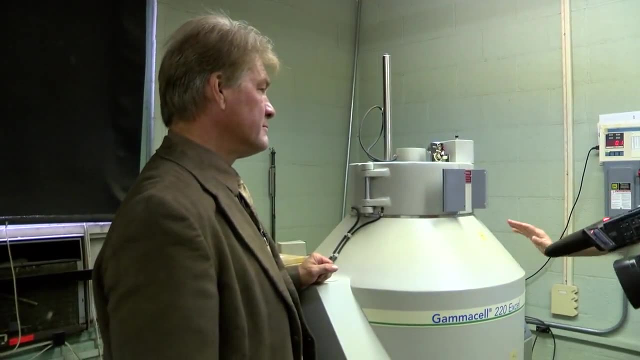 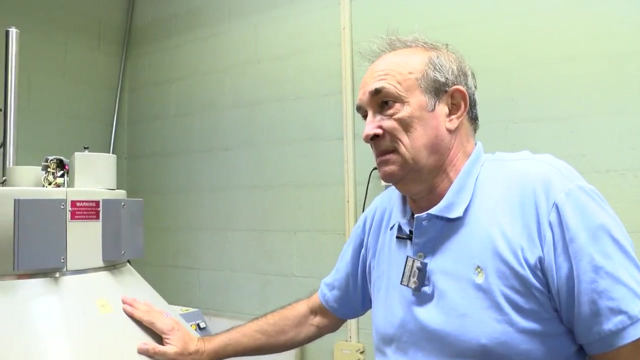 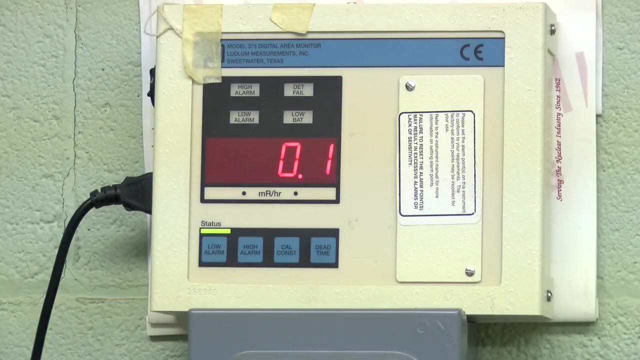 Okay, You can't actually like put your hand in where the radioactive source is? Yes, And the most important is that the lead stops all radiation coming from this machine. Right, This is a special room with a special reinforced floor, special steel platform, because, literally, 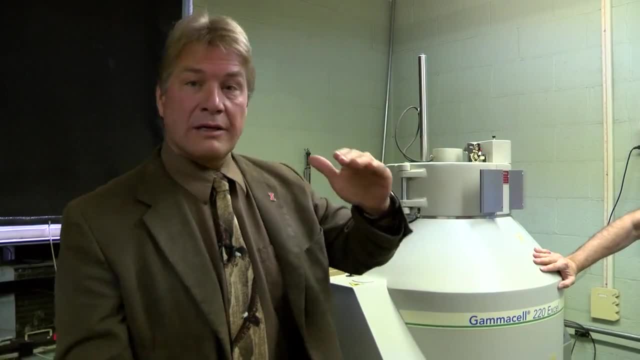 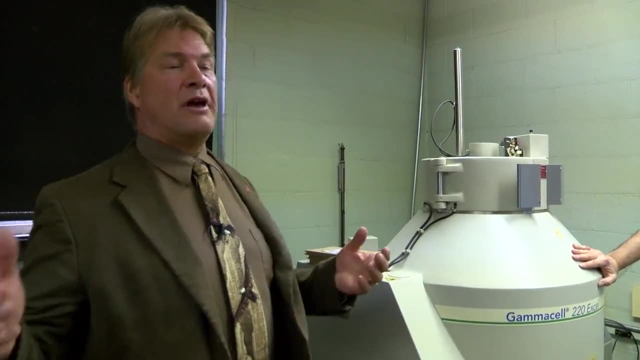 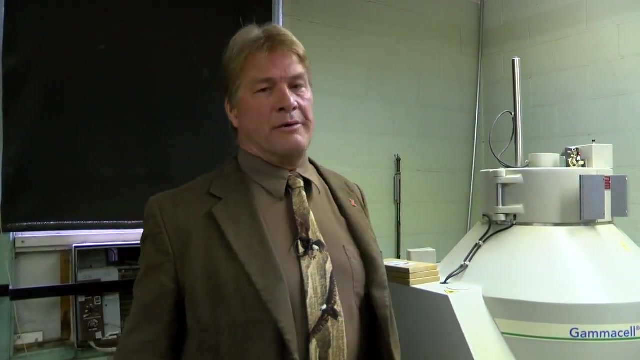 we have this thick of lead on all sides, underneath and around this, And lead is heavy, So this room is very special, And we also have, of course, all sorts of safety guards and automatic alarms and barred windows- although in reality that's a little bit silly, because I can't imagine anyone lifting.